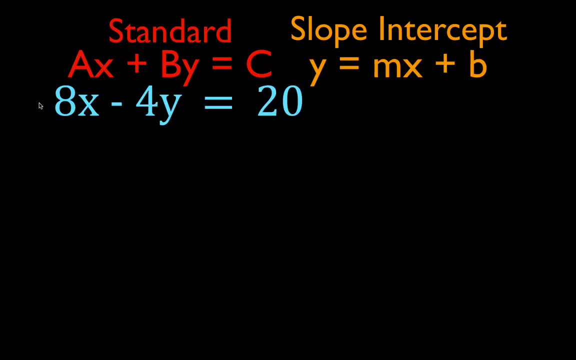 equals mx plus b. That means, in order to convert this equation to the slope-intercept form, we need to move everything over to the right-hand side of the equation, the right-hand side of the equal sign except the y. Now, in order to do this, we're going to follow two pretty 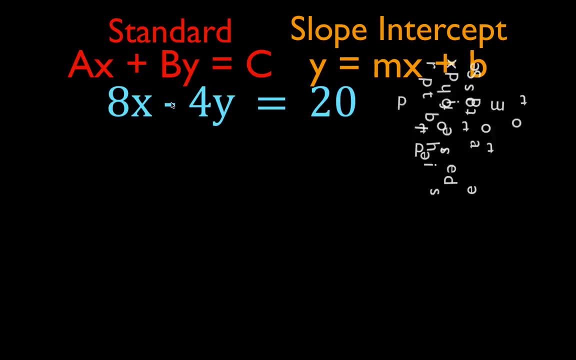 simple steps. The first step is this: This is the first thing you do: You always add the opposite of the x term to both sides. This is the x term: 8x. Opposite of 8x is is minus 8x. I'm going to add minus 8x to both sides. 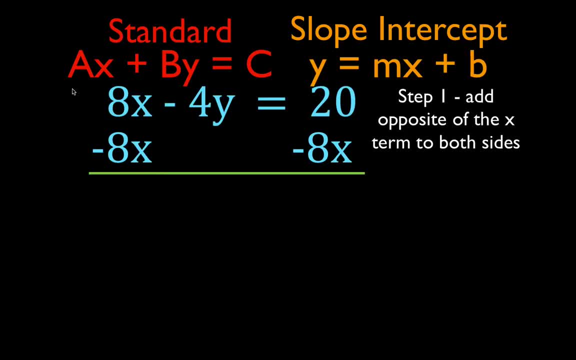 When I add minus 8x to both sides, I already have a positive 8x on the left hand side, so the 8x's cancel. I'm left with simply minus 4y. Don't forget your minus signs. Bring down the equal sign. 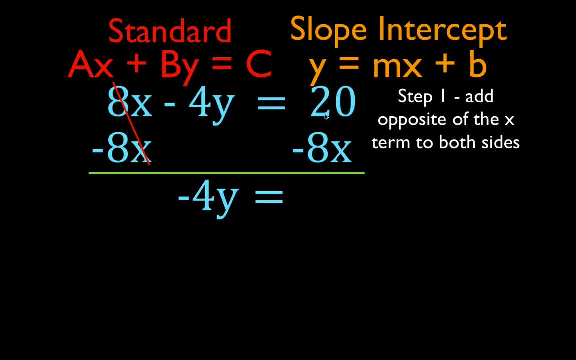 Now I'm gonna add minus 8x and 20.. Minus 8x plus 20 or 20 plus minus 8x is not 28x or 12x or something like that. These are not like terms. Minus 8x plus 20. 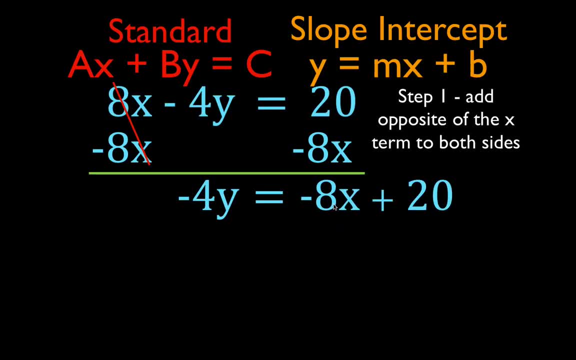 is simply minus 8x plus 20.. I wrote the x term first in front of the 20 because, as you can see in the slope intercept form, it's y equals mx, the x term and then the number, without the x or y. 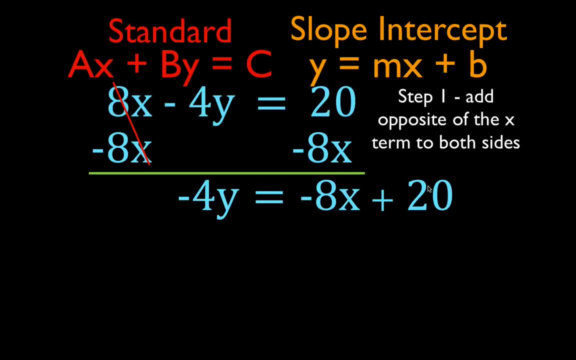 Now, that's the first step we have completed. We're going to do now the second step. The second step is simply to divide by the number that's in front of the y. The number that's in front of the y is minus 4.. 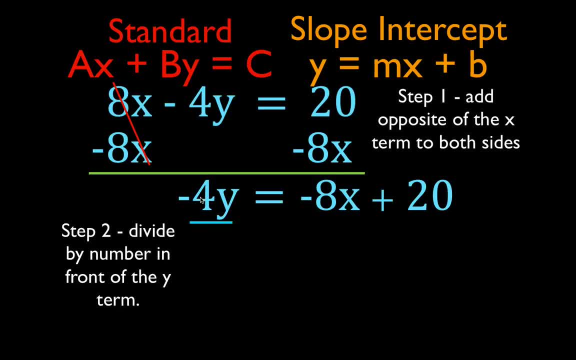 So I'm going to divide each of the terms, the whole equation, by minus 4.. Minus 4,, minus 4, and minus 4.. Minus 4y divided by minus 4.. The minus 4's cancel. 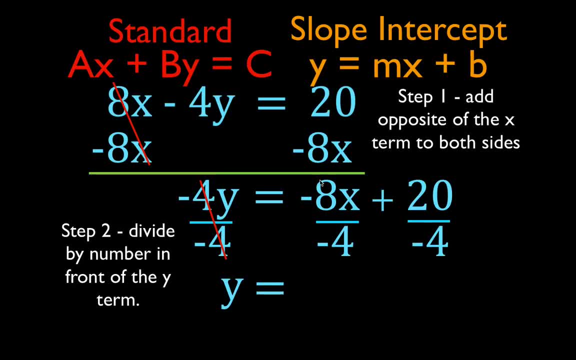 You're left with y, Bring down the equal sign. Minus. 8x divided by minus 4 is simply 2x. 8 divided by 4 is 2.. A negative number divided by a negative number is a positive number. 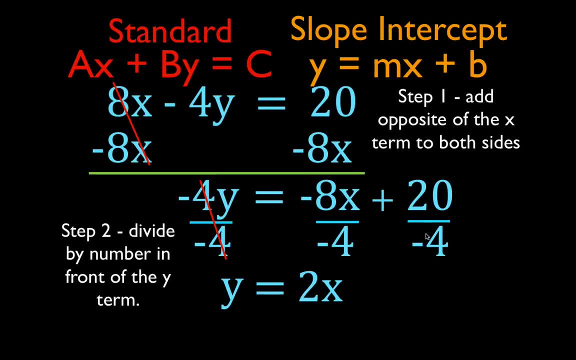 Keep the x. Now I'm going to divide 20 by minus 4.. 20 divided by minus 4 is minus 5.. That is the equation in the slope intercept form. y equals mx plus b. m is the slope, The slope is 2.. 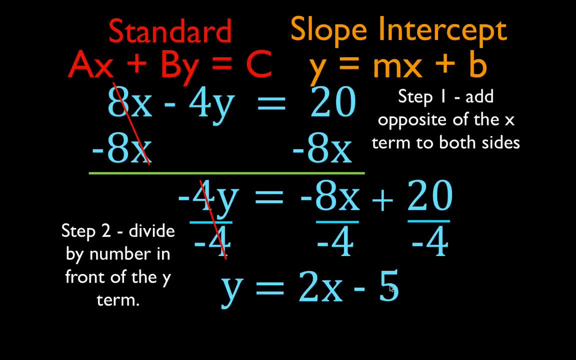 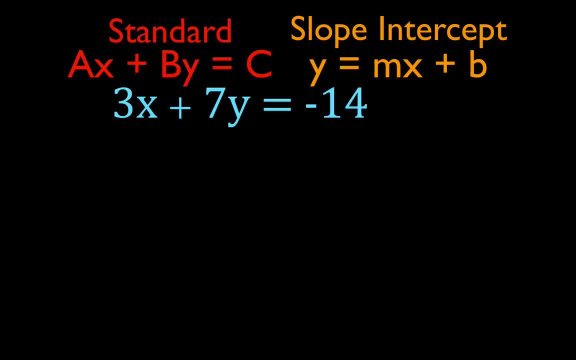 b is the y intercept. The y intercept for this equation is minus 5.. Alright, now we're going to do a couple more, We're going to go a little faster. Same two steps. Add the opposite of the x term, The x term is 3x. 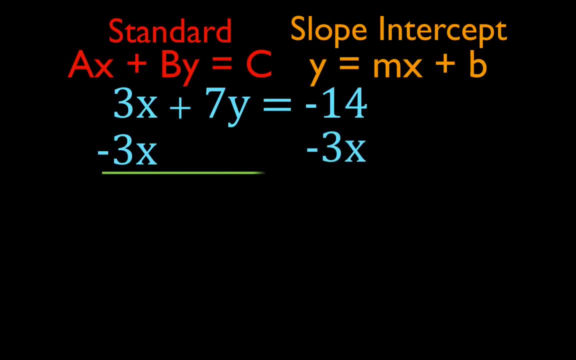 The opposite is minus 3x, The 3x cancel. You're left with 7y equals minus 3x, minus 14.. Step 2. Divide by what's in front of the y, That's the 7. Divide, divide, divide. 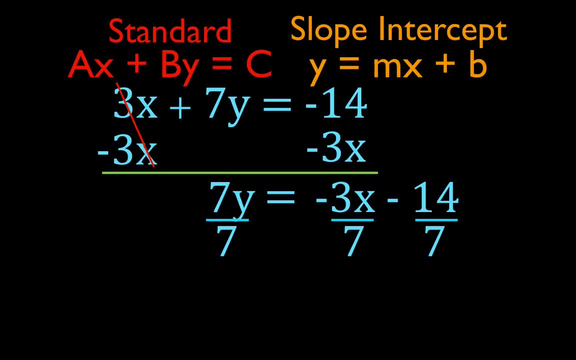 7, 7, 7.. Minus- excuse me- 7y divided by 7 is simply y, The 7s cancel. Now we're going to bring down our equal sign. Now, here you can see, we have minus 3x divided by 7.. Minus 3x divided by 7.. I'm going to leave it as a fraction. 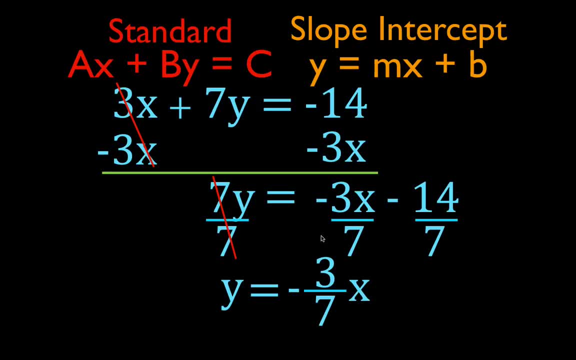 I just get minus 3, 7s x, and then 14, or minus 14,. minus 14 divided by 7 is minus 2.. That is the equation in the slope intercept form. y equals mx plus b, b is minus 2.. The slope is minus 3 sevenths. Don't forget your negative signs. 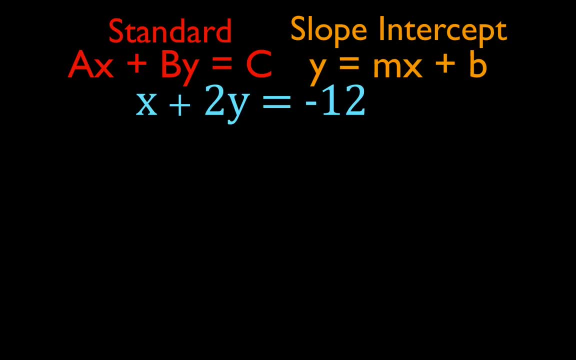 Next one: We are going to add the opposite of the x term. Well, the x term is x or 1x, so we are going to add minus x to both sides. When you add minus x to both sides, the x's cancel. 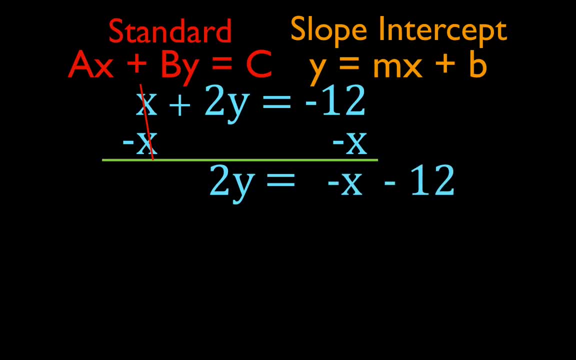 You are left with: plus 2y equals minus x minus 12.. Now we are going to divide by the term that is in front or the number that is in front of the y, That is, a 2,, a 2, and a 2.. The 2's cancel. 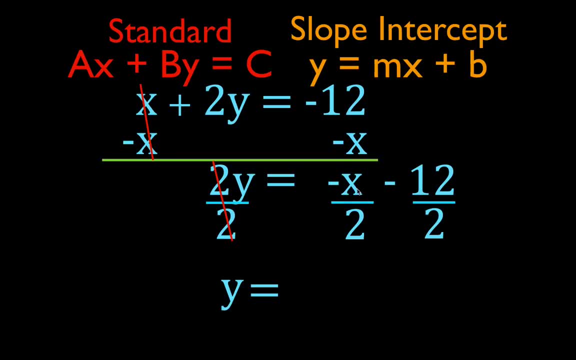 You are left with y equals. Now this is minus x. There is actually a 1 in front of here, We don't write it down. So minus x, minus 12.. Now we are going to add minus x to both sides. When you add: 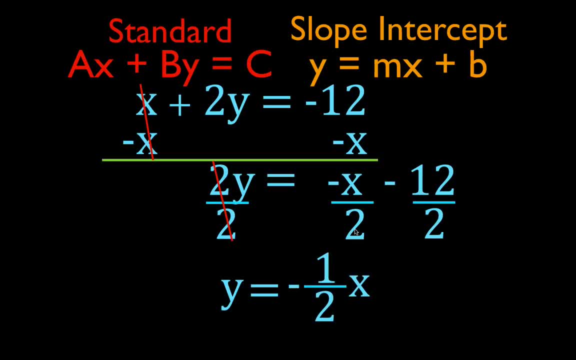 minus x divided by 2 is minus 1, half x. And then minus 12 divided by 2 is minus 6.. This is the equation in the slope intercept form: y equals mx plus b, b is minus 6.. m- the slope, is minus 1. 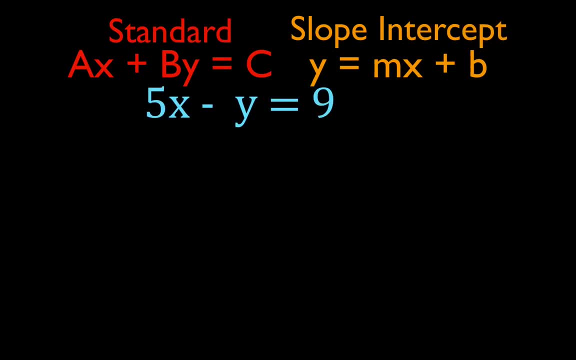 half One more. Now we have 5x minus y equals 9.. We are going to add the opposite of the x term, Once again the x's cancel. We are left with minus y. y equals minus 5x plus 9.. Now this may look like it is in the slope intercept form: y equals mx plus b. 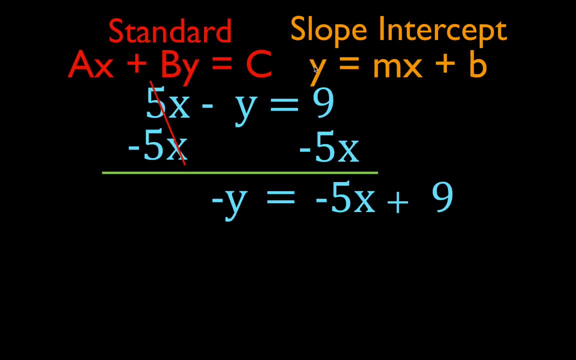 But this is not y minus y, It is just y And here we have minus y. So in order to get rid of the minus, there is actually a minus 1 here in front of the y. So we are going to divide the whole equation. 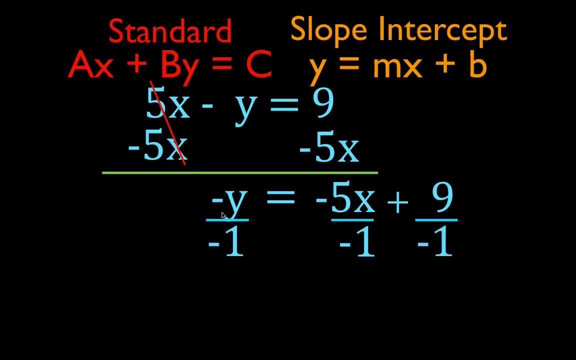 by minus 1.. Minus 1.. Now, minus 1y. Divided by minus 1 is just y, because the minus 1's cancel Equals minus 5x. divided by minus 1 is simply 5x. 5 divided by 1 is 5.. 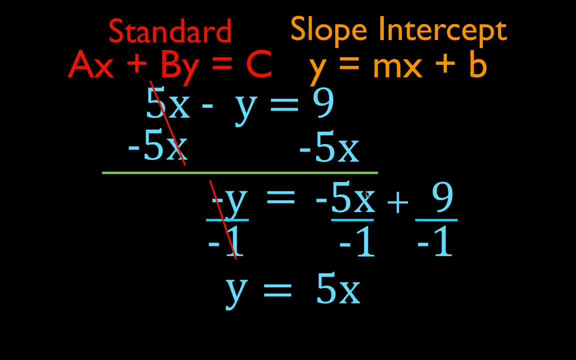 And negative divided by negative is a positive. We bring down the x again: Minus 9.. Okay, so that is the slope intercept form. y equals mx plus b, b is minus 9.. The slope is 5.. Okay, so there you go. We did four different examples. I tried to cover a whole range of possibilities. 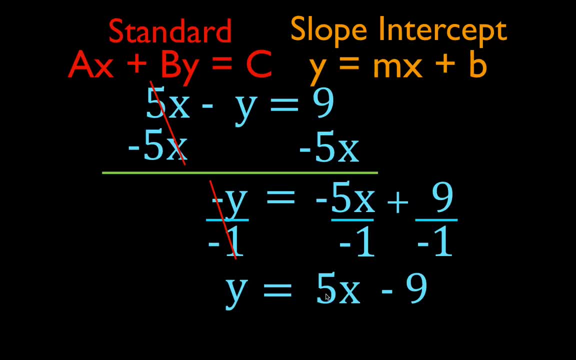 I hope you found that helpful. Do those steps. Add the opposite of the x, Divide by the number that is in front of the y. Thank you very much for watching. I hope you found that helpful. If you found that helpful, you can do one or all of the following three things. 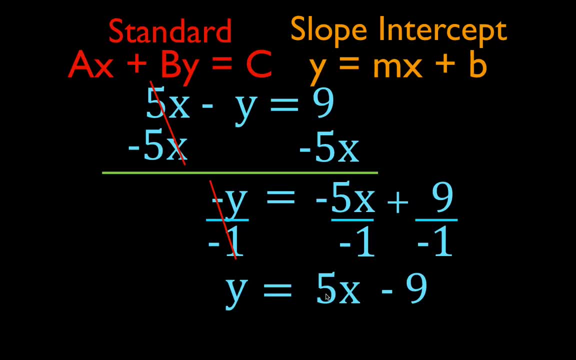 Subscribe to my channel, Get all my excellent physics, chemistry and math videos. You can give me a thumbs up for this video And you can leave me a nice, positive comment in the comment section below. Thank you very much.